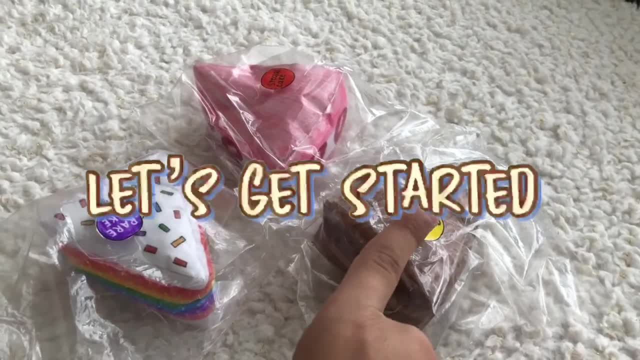 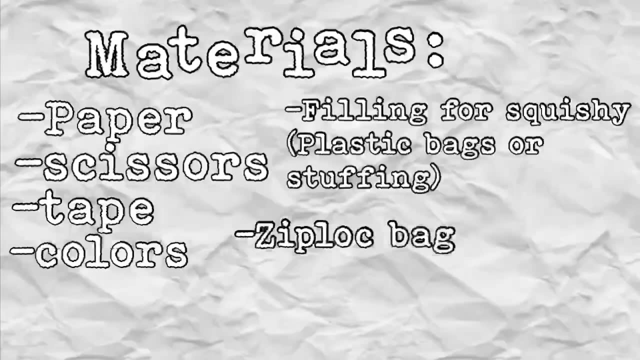 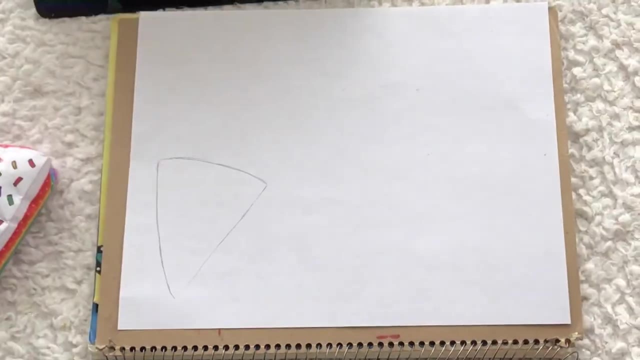 totally keep on growing from here. So, yeah, let's just get on to the tutorial. Okay, guys, the first step is to make the top of the cake. So you're gonna make a triangle shape And you see me here tracing my other cake, because I want all my cakes being the same size. Then take your marker. 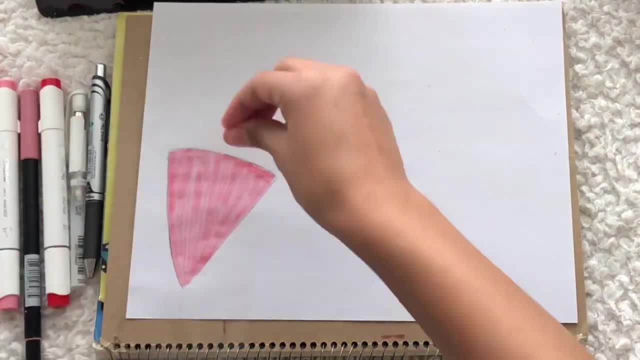 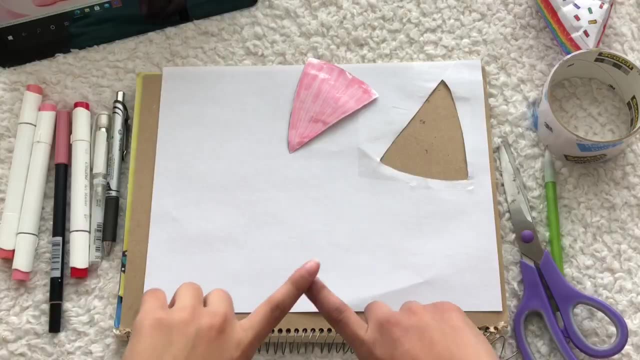 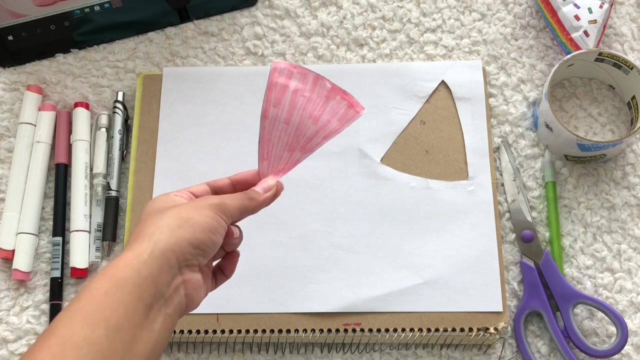 and color it whatever you want- I'm gonna do a light pink because I'm doing a strawberry short bay flavor- Then cover it with tape and cut it out. Okay, guys, now that we have our top of the cake, we're gonna now place it on the piece of paper right beside our first triangle that we 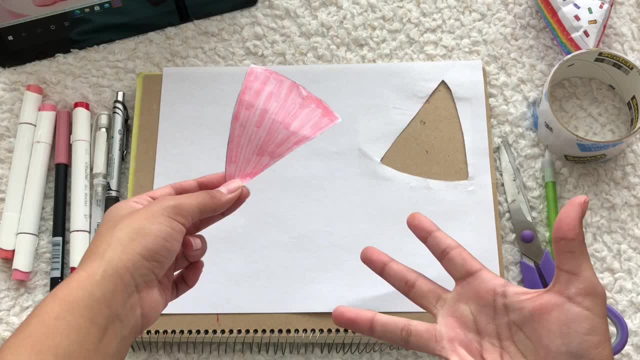 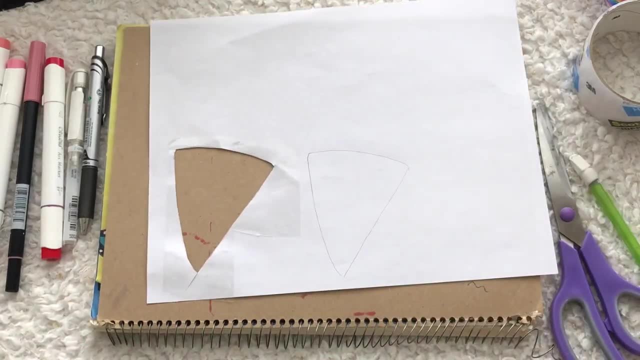 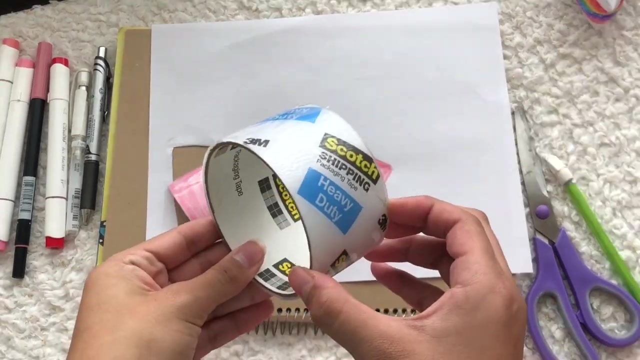 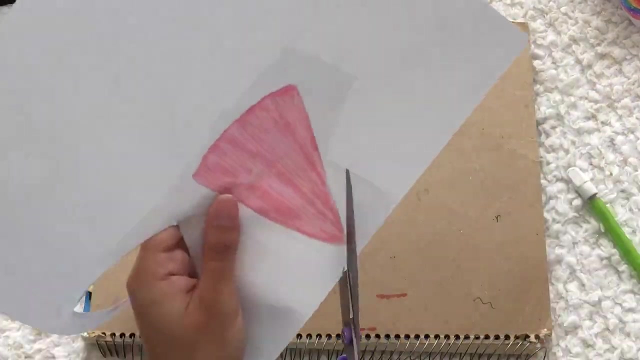 cut out, Trace it out and color it If you're gonna add any color to the bottom and cut it out again. So we're gonna have two triangles. Now just get your tape again and laminate your second triangle. Okay, guys, ignore the shower noises in the background. My sister decided to leave the shower while I was filming. 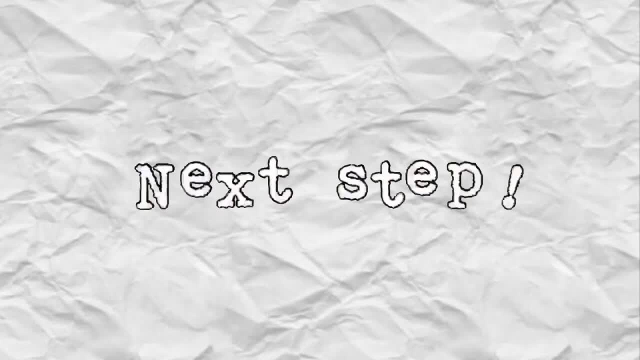 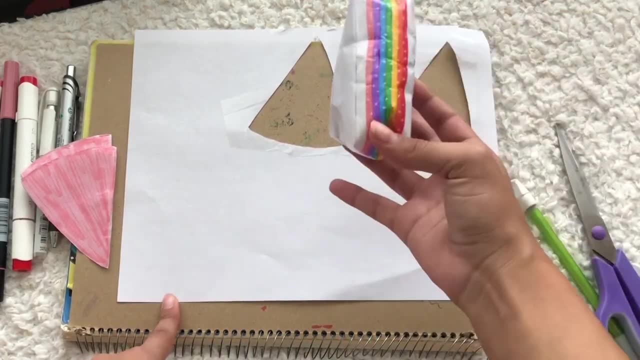 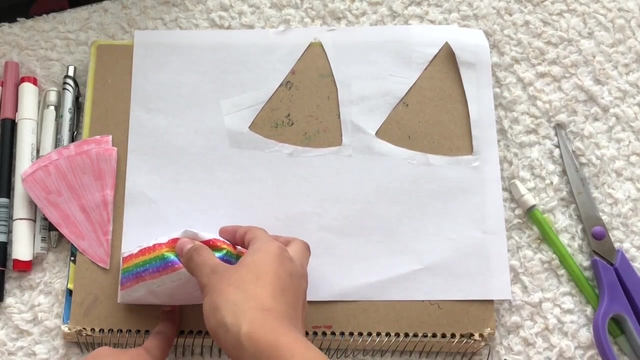 But anyways, now we're gonna put these to the side right here And we're gonna take this edge of the paper And since I already made another one, you can like measure it out if you're making several ones. So just decide on the width of your mini cake. So I would just trace right here and just put a. 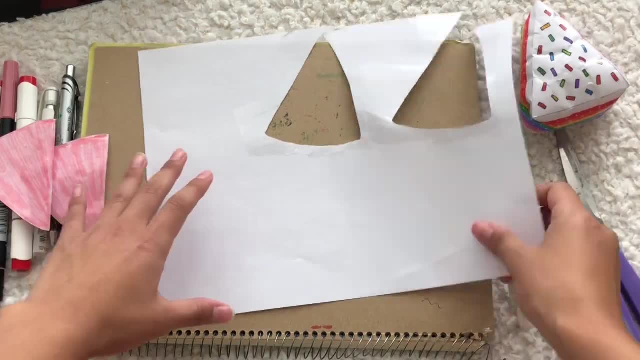 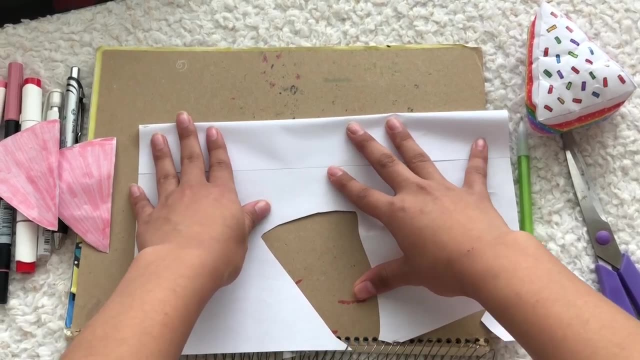 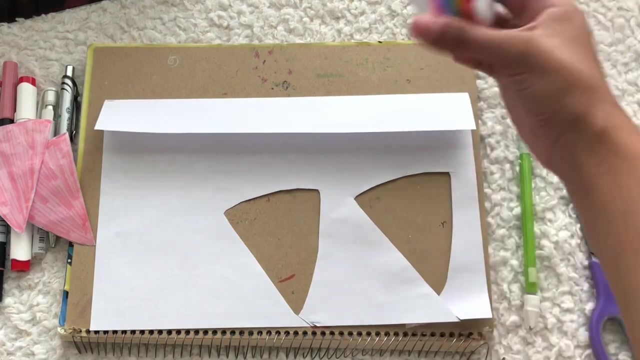 little mark. So then, for the line to be straight, I always just fold the paper as straight as I can. Ummm, Like that, And for me the funnest part is to like design the side, because, as you can see, it's like very colorful. 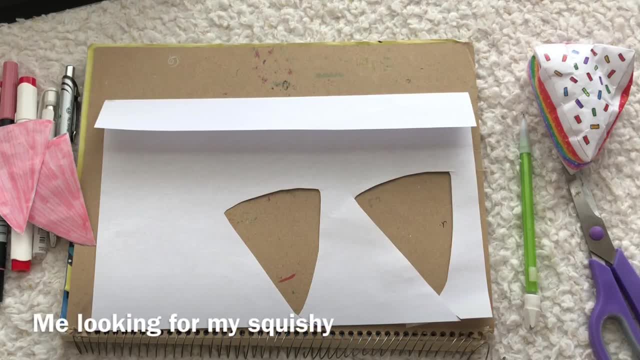 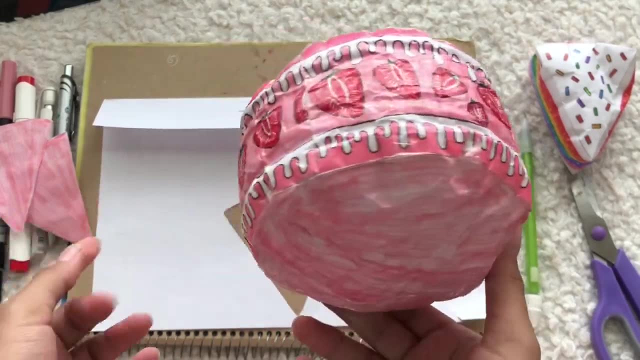 depending on the cake you're doing. So I have this really old cake that I made like a couple months ago and it is this strawberry cake And basically, as you can see, like the side it has like strawberries and whipped cream, little drips, And I just think that's gonna be our side of our cake. 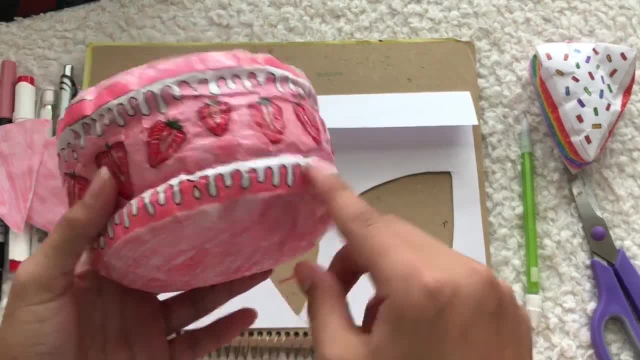 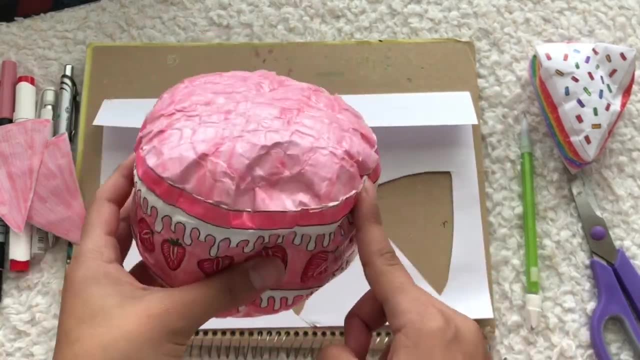 So we're gonna put this aside. We're gonna wrap this around strips and i just think it's like super fun and this squishy is so like slow rising and i'm kind of recreating this, but like in a little slice, but with like more detail, probably like chocolate or 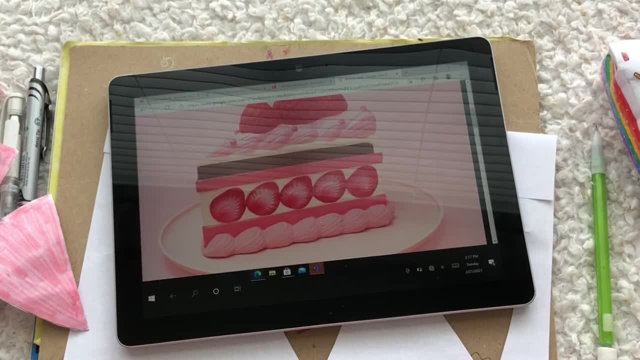 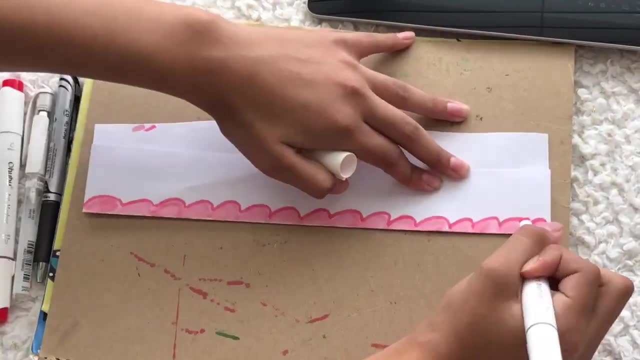 something and i'm gonna try to recreate the side of this. i bloom cake to my mini cake, so now i'm just coloring the sides and i made these little light pink dollops on the bottom half of the cake. and i really like how i did the strawberry slices on this cake, because on the other one i like didn't. 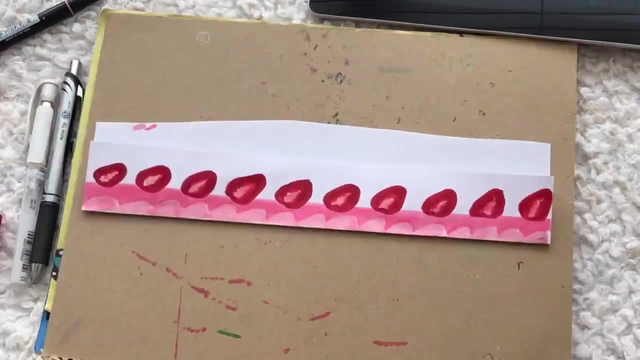 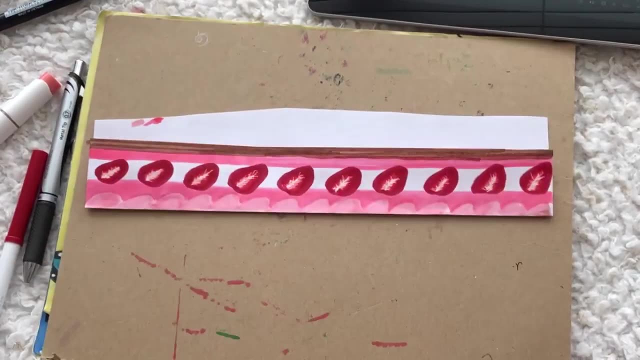 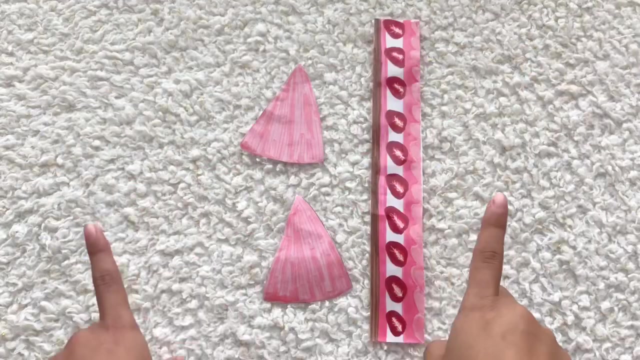 have my white detail gel pen, so i think this one turned out really cute and i kind of like shaded it a little more and, yeah, i just added two more layers to the top. all right, guys, i've cleared this space a little bit so we can get on to this next part. 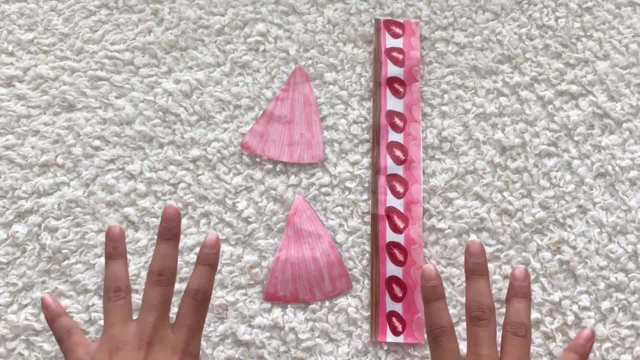 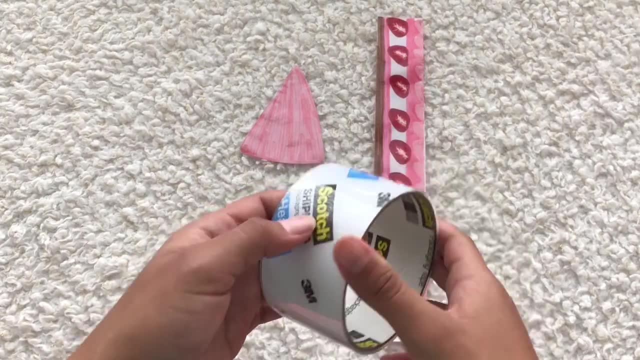 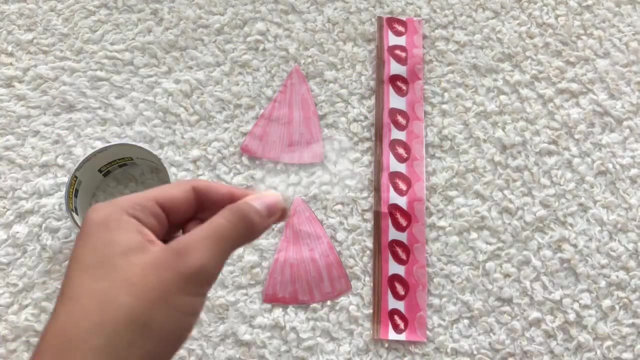 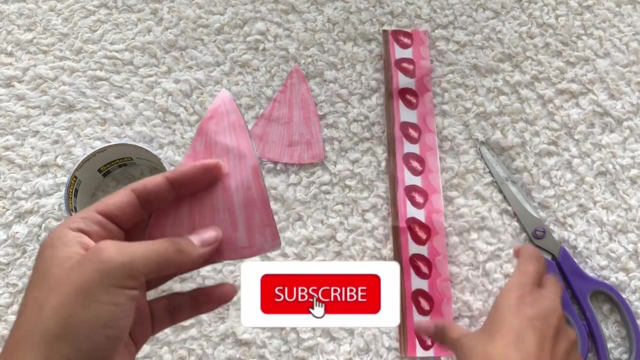 so we should have three pieces of paper in total right now: the top, the bottom and the side. so we're gonna take little pieces of tape like this. we're just gonna get a little piece- i get pieces like this big- and then just cut them in half. we're gonna take the top and the side and 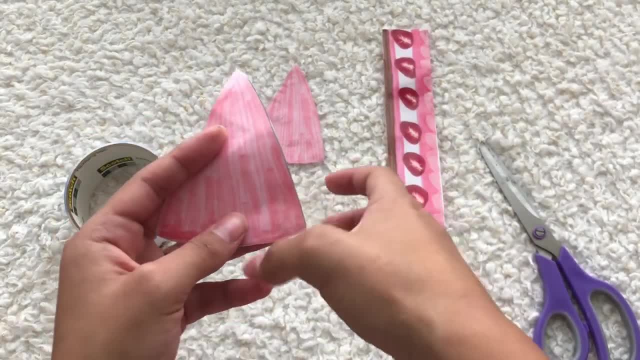 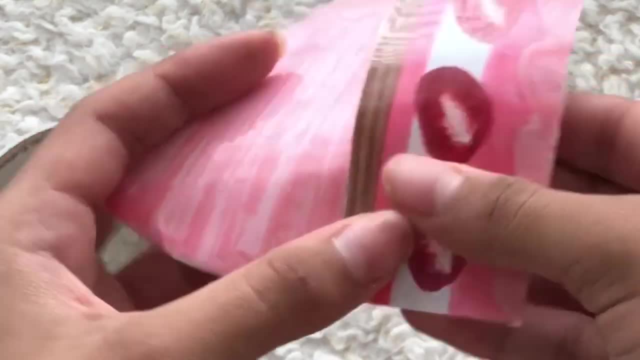 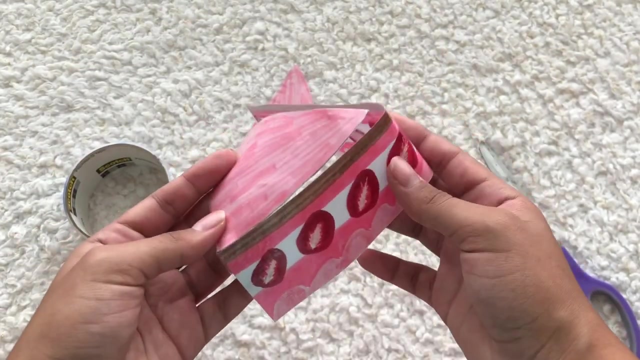 just put a little piece of tape on any side of the little triangle. it doesn't really matter where you put it first, and just tape the side like this: make sure it has no holes like in the middle. so just start taping your little side of the cake around your triangle. 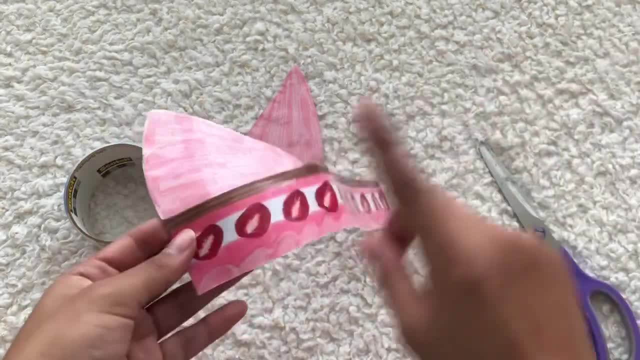 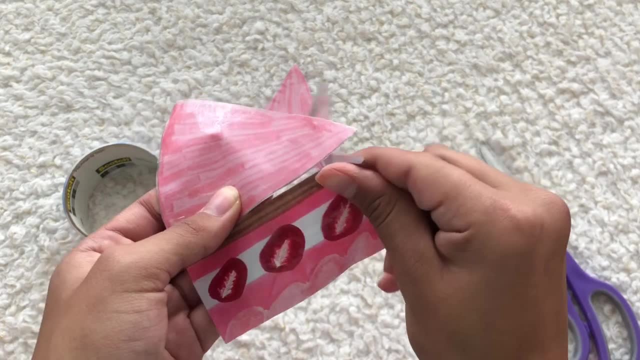 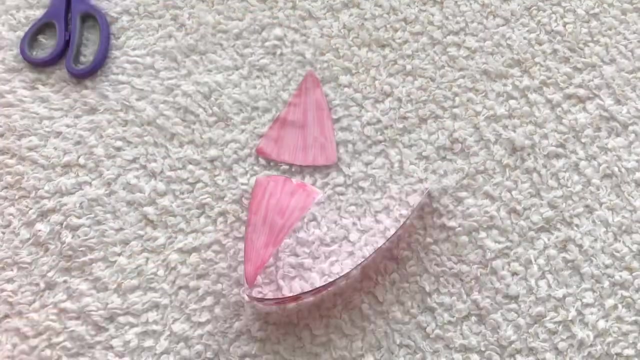 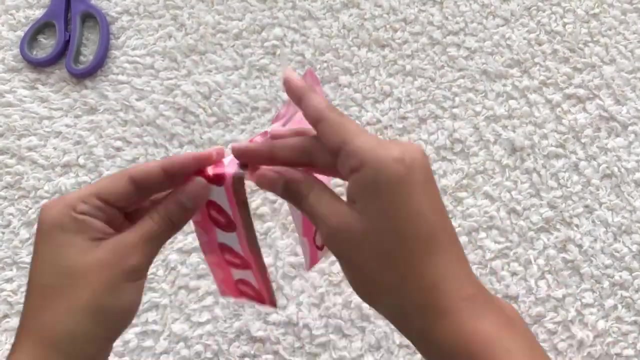 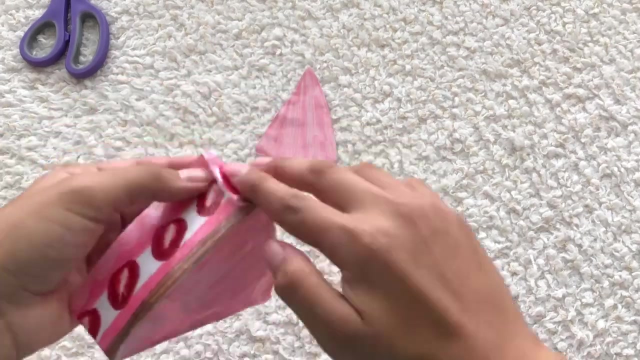 and you'll eventually come back to here. you can overlap it with the extra paper or cut it off, and when you get to these kinds of corners, just fold the paper like this so it can have the shape of the cake. okay, so this is how it looks so far. i think it looks so adorable and i can't wait to squish it. 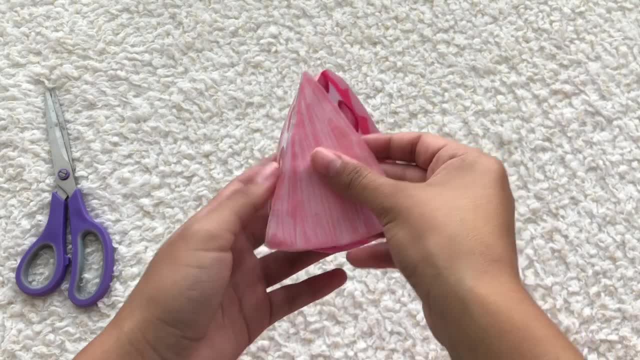 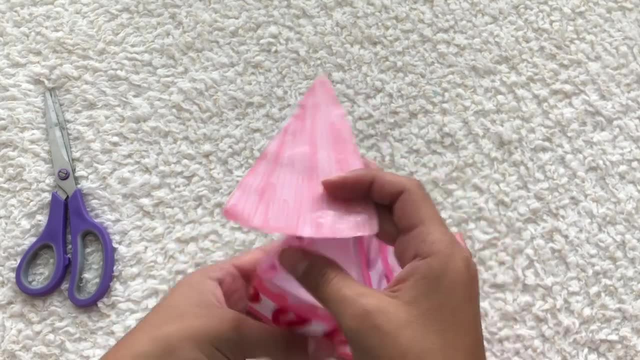 but we still have one more side to tape. so now we're just going to take our tape again and tape all the sides except one. you can leave any side open, preferably the smaller one, so it's easier to tape at the end when you're filling it. so now you're just gonna tape it and fill it up and then 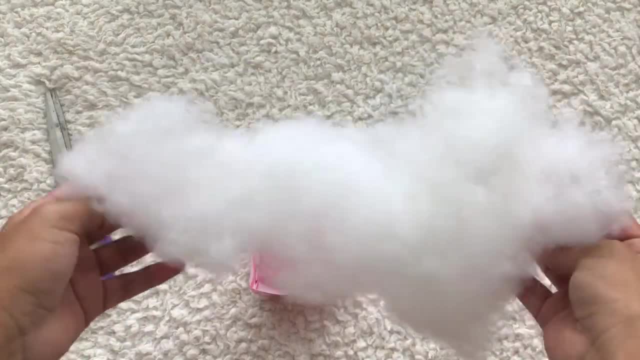 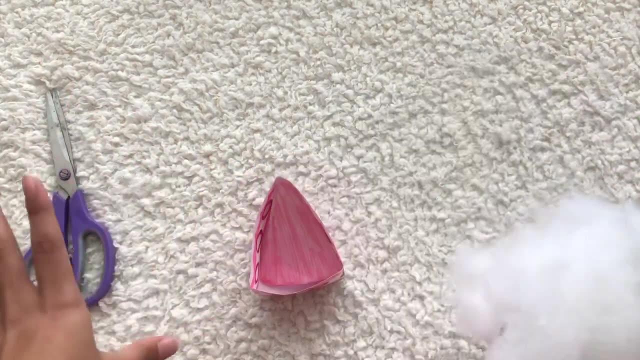 fill it up. i'm gonna be using this stuffing. it's called polyfill and you can get it at walmart, but you can also use plastic bags or cotton balls or maybe newspaper if you don't have anything else. but i recommend this because it's the best to use. 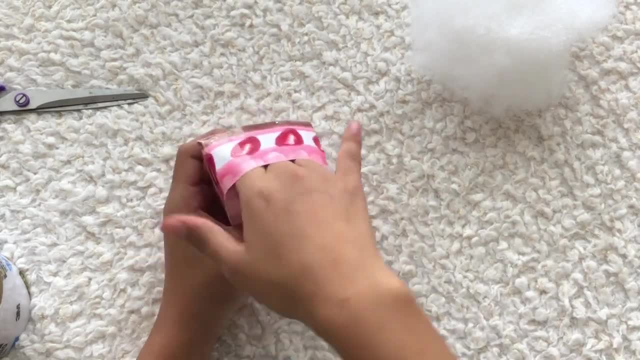 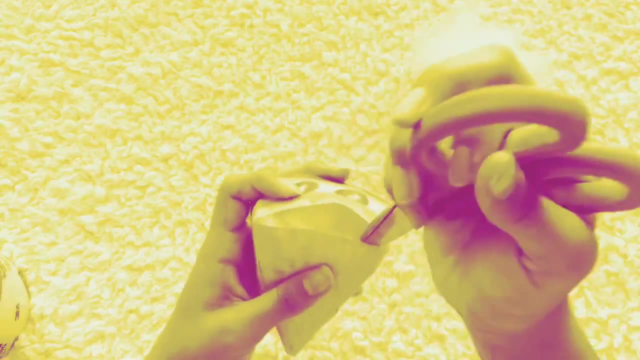 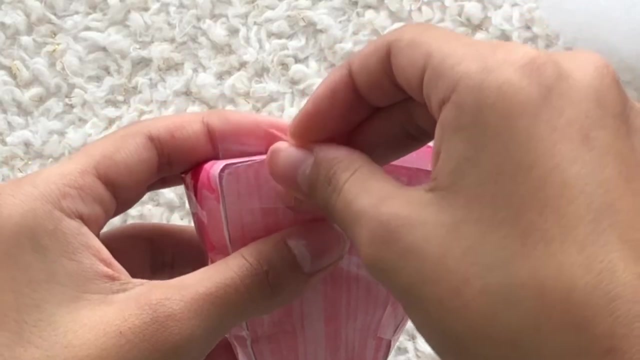 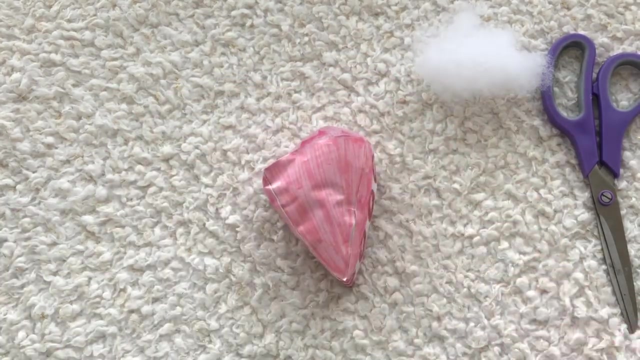 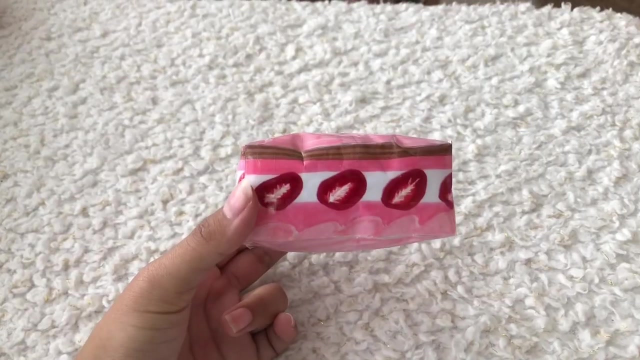 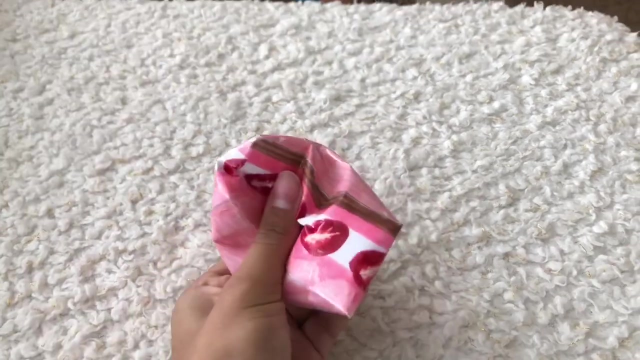 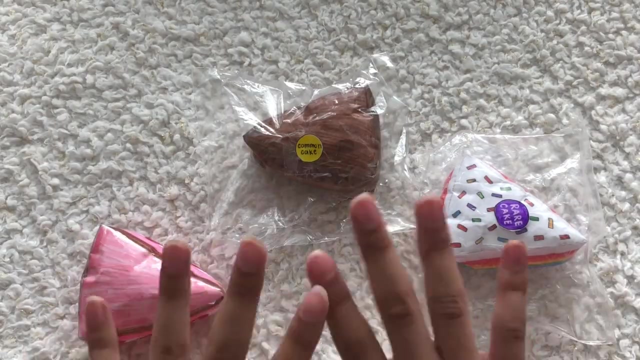 okay, now we're just gonna tape it shut where we just filled it up like this. okay guys, so this is how the paper squishy turned out. i think it looks so cute and it's super squishy. okay guys, now i'm gonna show y'all how to make this super easy, clear packaging for your cakes. 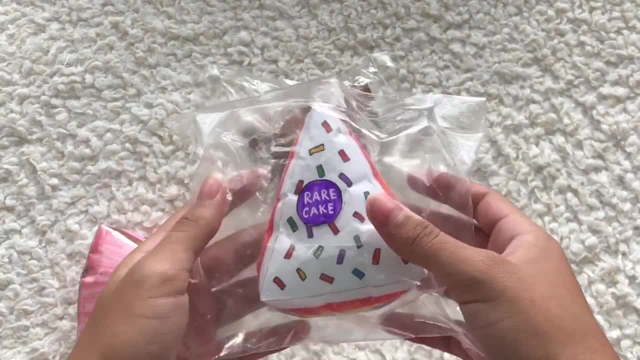 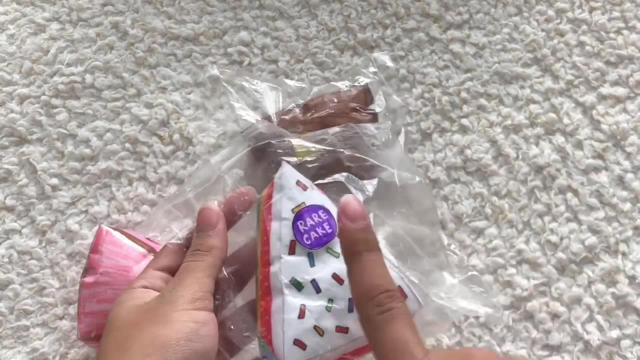 it's just this little square um plastic bag for your squishies, and i just think it looks super cute with a little sticker. you could put any kind of sticker, but i put mine as like the rare cake, and then this one's the common cake. so let's get started. 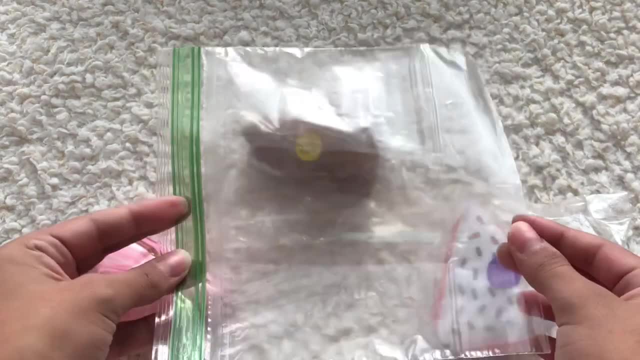 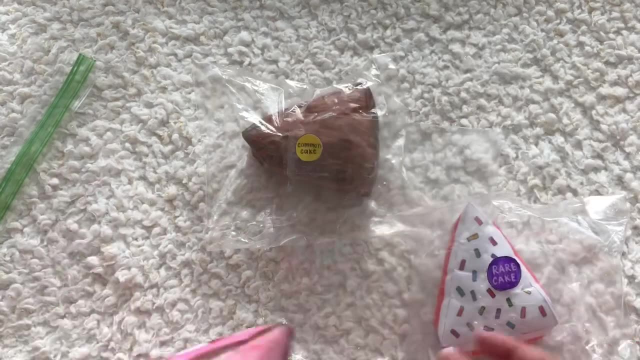 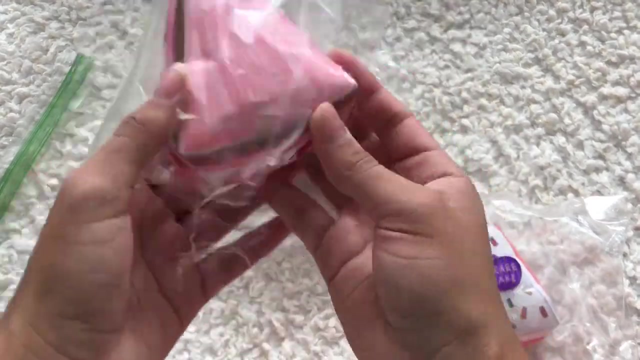 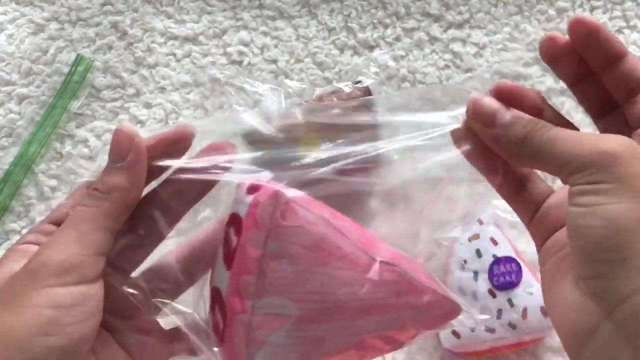 okay, we're gonna take this ziploc bag and cut the little green part off. now we could just put this part to the side, and we're gonna take our squishy and just put it in right here, like that. and um, then you're gonna take some tape and start taping the edges shut. 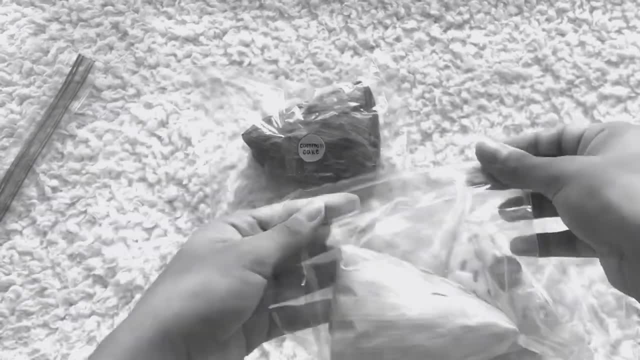 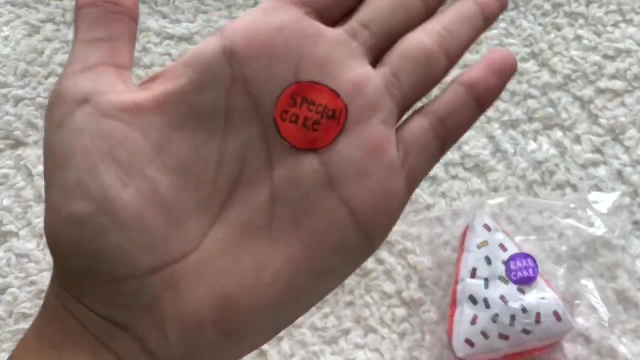 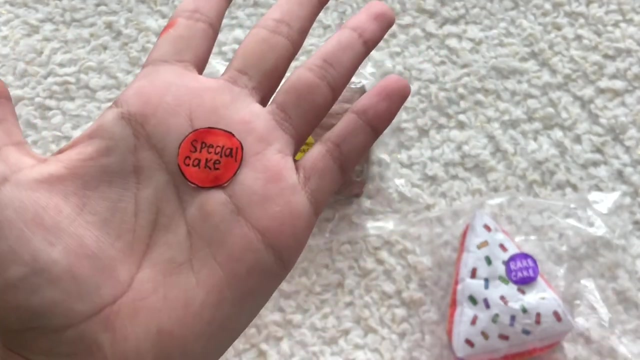 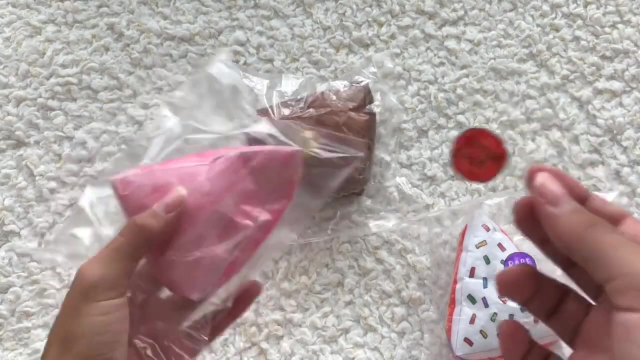 and right here i drew this little circle and i put special cake on it, because that's what it has on the list for my little blind bags that you guys probably saw from yesterday's video. you're just gonna put a piece of tape like this and put it on top of your bag, just like that, and